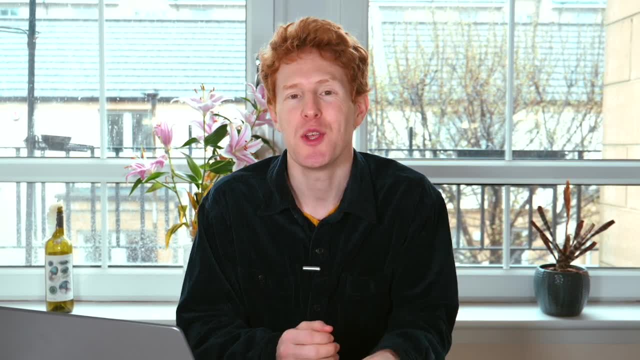 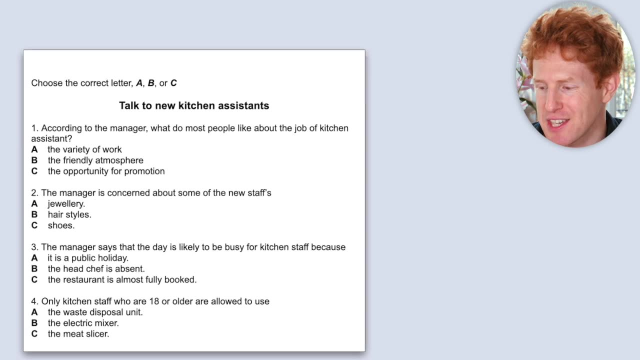 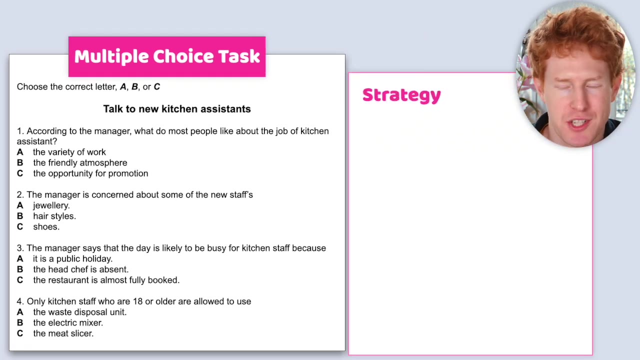 Hey there, welcome back. In today's lesson. you and I are going to do a multiple choice task for IELTS listening. Let's have a look at the task we're going to do. It's this one, a multiple choice task. What's going to be our strategy? Well before the recording starts. 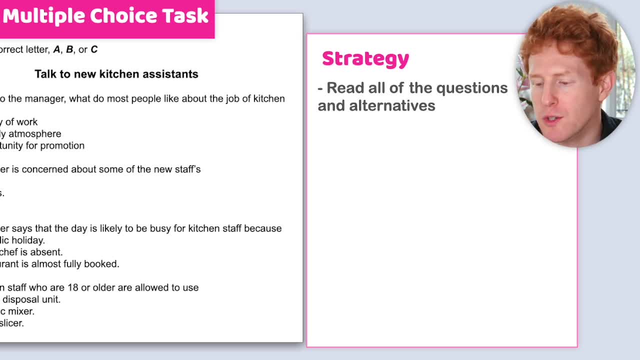 you've got a couple of moments to read all of the questions and alternatives. Now, while you do this, I think it's important that you underline key words in both the question and the alternatives. Now, once you've done that, for all of the questions, return back to number one and start to 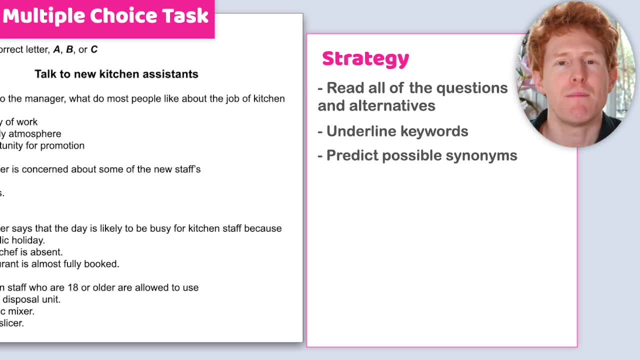 predict possible synonyms. Remember, synonyms are words or phrases that mean the same thing. Also, while you're doing this, I suggest that you predict some possible tricks that examiners might play. We'll be doing this together, so I'll show you what I mean in a second. 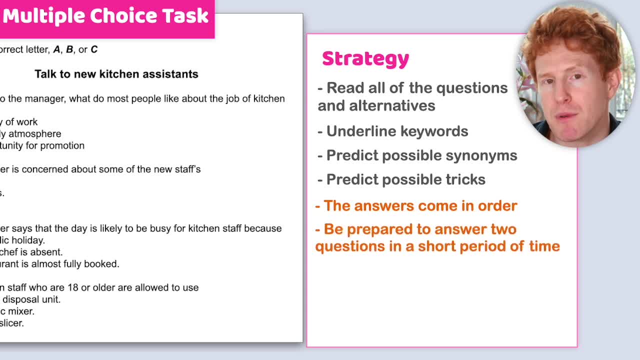 Remember the answers come in order. You need to be prepared to listen to two questions in a short period of time. You're going to circle the answers on the question paper and transfer these answers neatly to the answer sheet at the end and practice writing the answer while still. 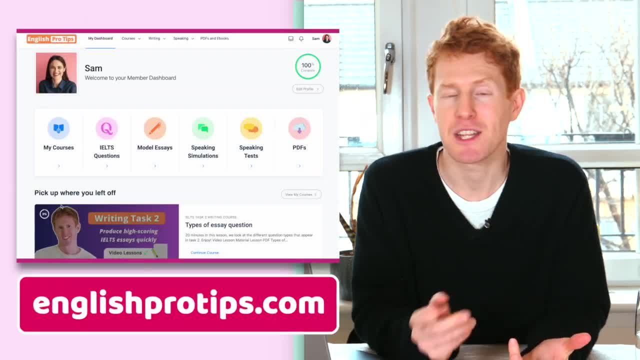 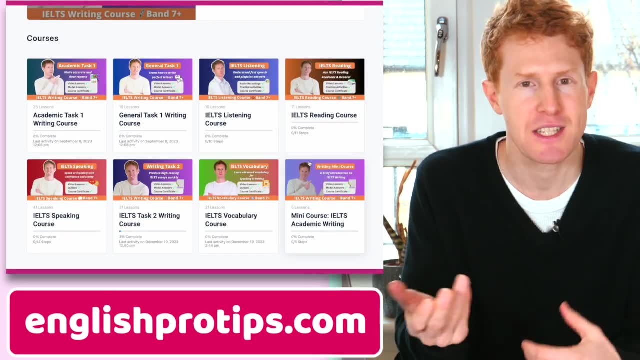 listening to the audio. Hey there, if you're enjoying this activity, then check out English Protipscom, where you'll get help for all parts of the IELTS test: the listening test, the reading test, the writing test, the speaking test. You can start for free at English Protipscom, See you. 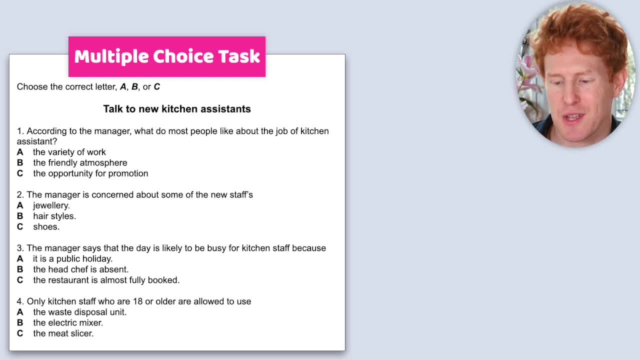 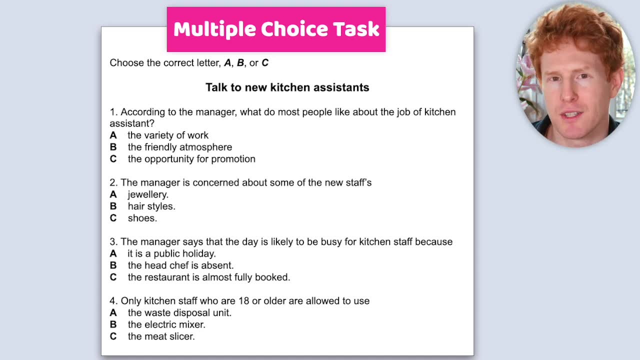 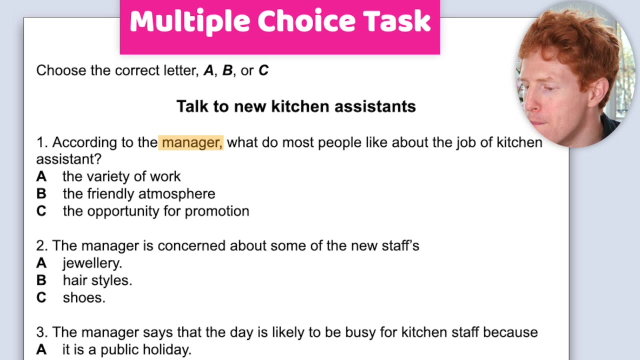 inside. Okay, let's do this together. So go to number one and begin to highlight words that you think are the key words. Let's do it together. According to the manager, what do most people like about the job of kitchen assistant? The variety of work, the friendly atmosphere or the? 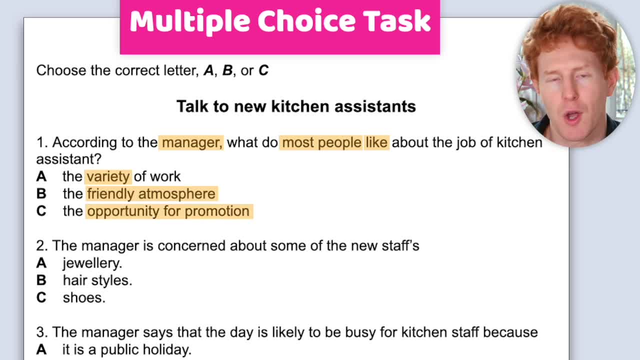 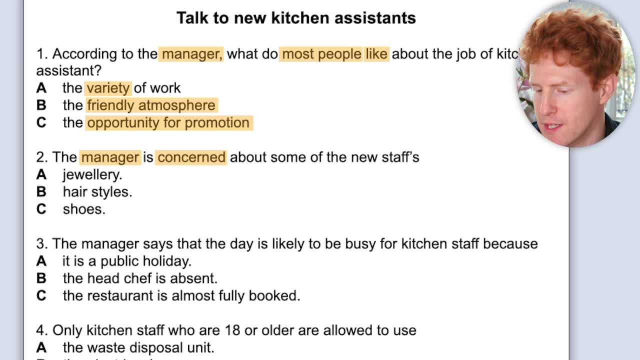 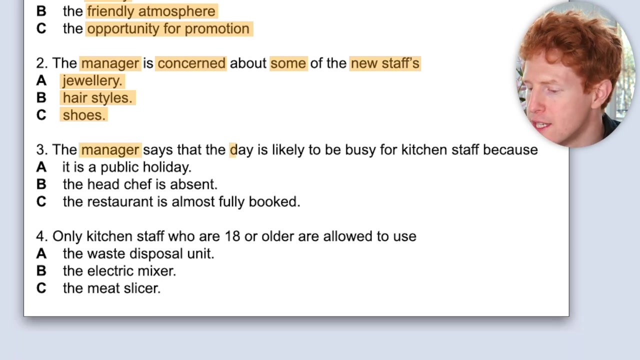 opportunity for promotion. Okay, number two: The manager is concerned. so concerned means worried about some of the new staff's jewellery, hairstyles or shoes. Okay, number three. The manager says the day is likely to be busy for the kitchen staff because 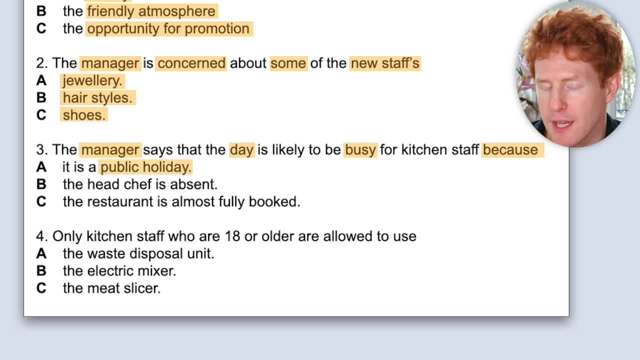 so we're looking for reasons. it is a public holiday, like Christmas or New Year's. The head chef is absent, so the main chef in charge of all of the other chefs and kitchen assistants is not there. They are absent. The restaurant is almost fully booked, so not fully booked. 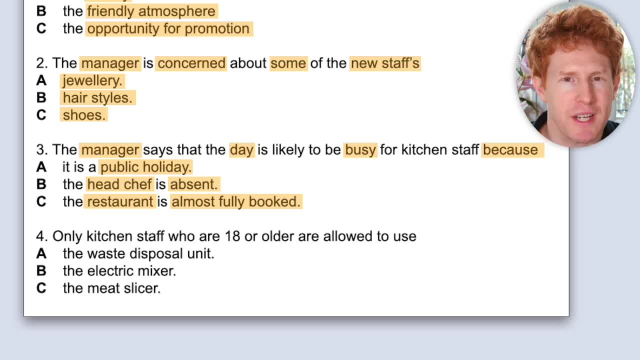 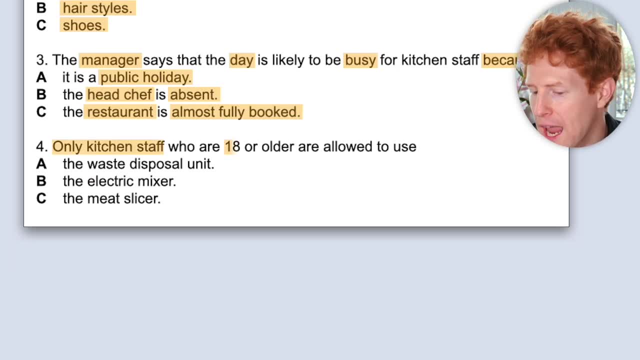 but almost fully booked. The manager says the day is likely to be busy for the kitchen staff, so not fully booked. That will be important. That's the kind of trick that an IELTS examiner can play on you. Okay, number four: Only kitchen staff who are 18 or older, so over the age of 18,. 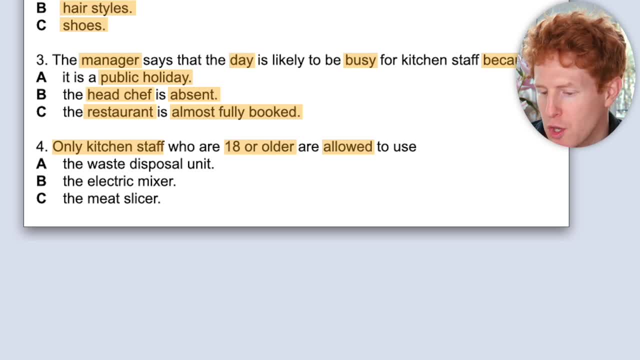 are allowed to, so permitted to use the waste disposal unit, the electric mixer and the meat slicer. So these are words that describe machinery in a commercial kitchen. So if we've still got time, we're going to go back to number one and we're going to think: 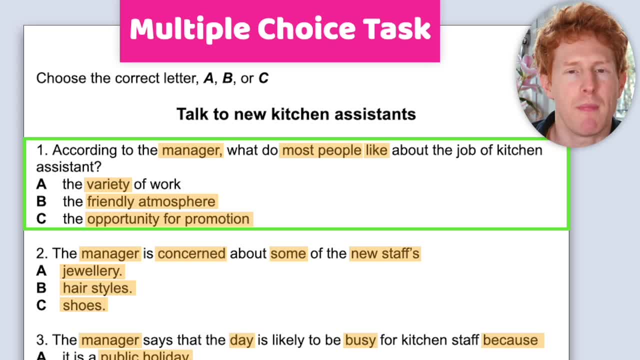 about synonyms for these words and phrases. So manager, well, we could say boss. most people, like many people, enjoy Variety of work. we could say something like many different roles, Friendly atmosphere, enjoyable ambience, opportunity for promotion, ability to go up the ladder. 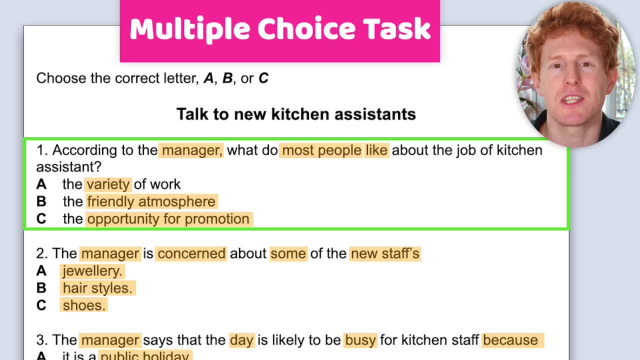 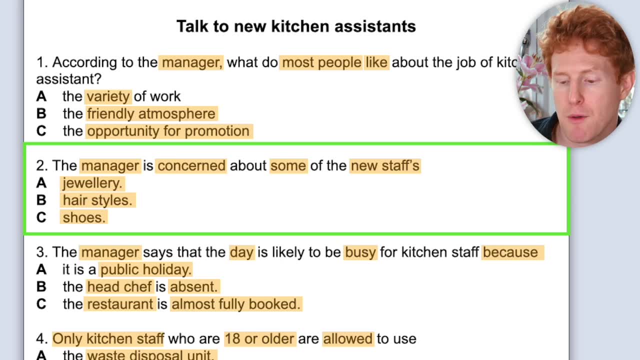 Okay, just think about these synonyms. By doing this, you're going to be engaging and learning more about the question. Then we go to number five. So if you've still got time, you're going to number two. Okay again, manager, we could have boss Concerned. we could have worried. 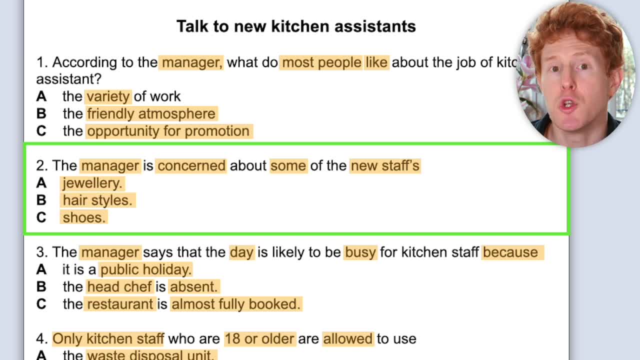 Some of the new staffs, so some of the new recruits. for example, Jewellery- well, there's not really a synonym for jewellery, but they might mention different jewellery like: be careful about rings or earrings. Hairstyles: maybe you need to wear your hair up in a bun so to avoid hair. 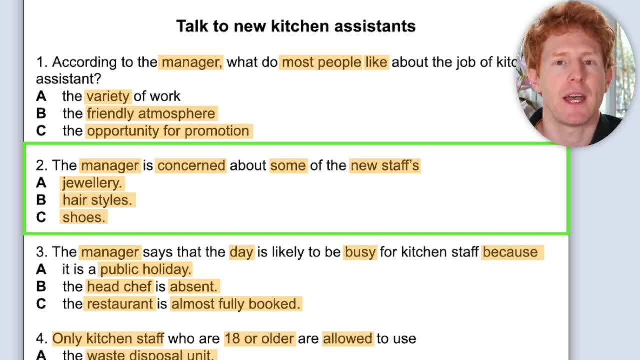 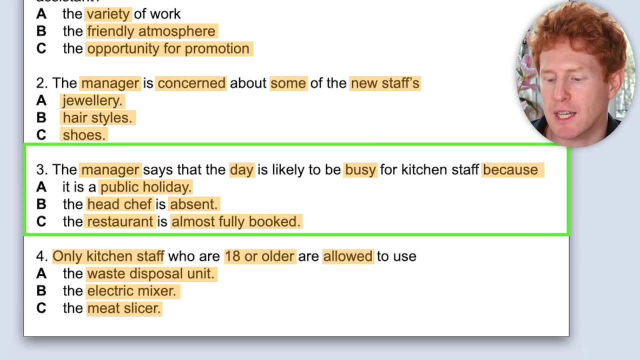 falling into the food. And then shoes. we might get different words for describing shoes, like suitable footwear or appropriate trainers. Number three: again, manager, we've got boss. The day is likely to be busy for kitchen staff because- So we might hear that for kitchen staff, you'll be likely to be. 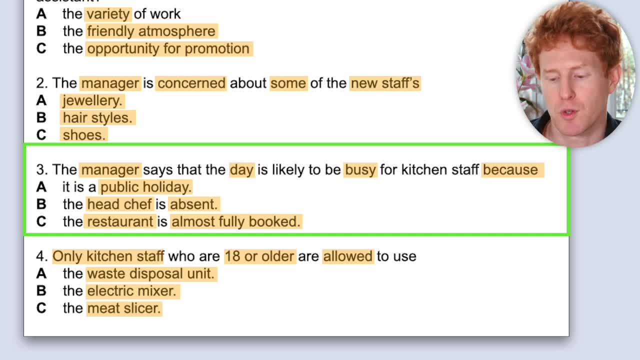 running around because of or for the reason of, And then we might get different words for kitchen staff. So we've got public holiday, So they might mention what holiday it is. like Christmas, The head chef is absent, So you might hear something like the main chef is not here, or 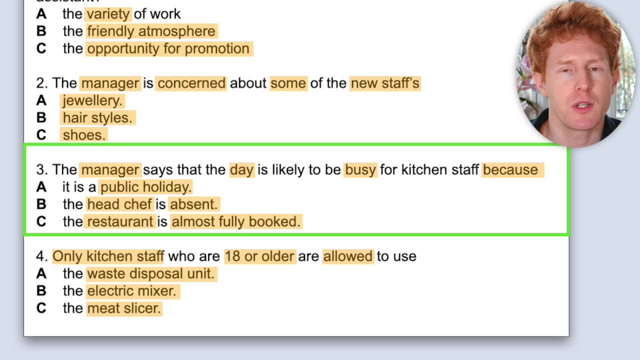 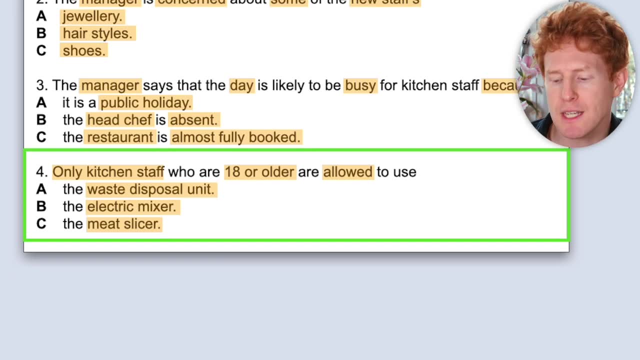 is on holiday, The restaurant is almost fully booked, So all the tables have been reserved. And then we go to number four. Only kitchen staff who are 18 or older are allowed to. So only kitchen staff who? or no kitchen staff. 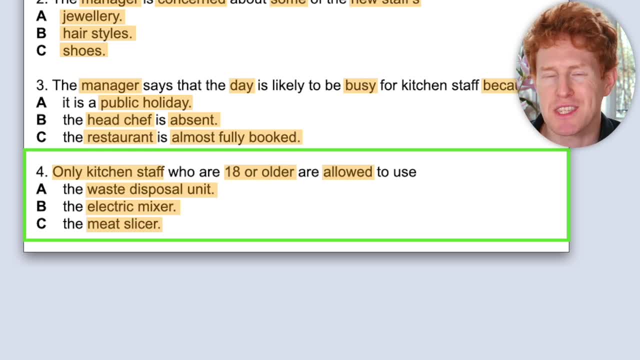 under 18 are permitted to. So you can see the way an examiner might play a trick on you. Instead of talking about people that are over 18, they might say: people who are under 18 are not allowed to do the same thing. Okay. And then we've got phrases like waste disposal unit, electric mixer. 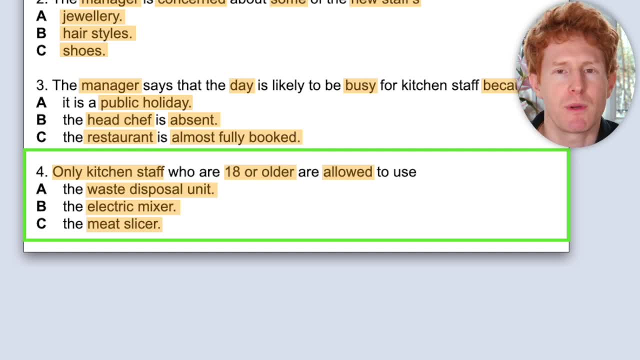 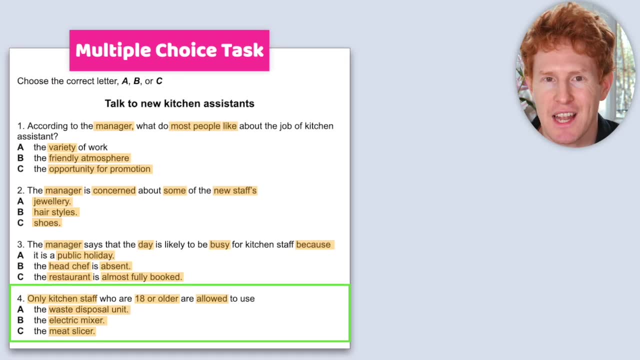 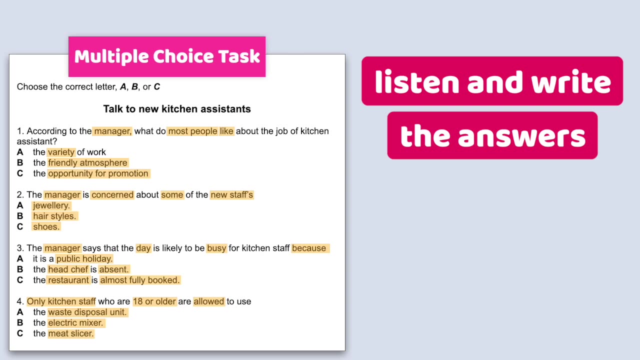 meat slicer. We're unlikely to hear synonyms for these words because they are technical words that describe machinery in a kitchen. Okay, Let's listen to number four. Listen to the recording and choose the correct answer. You can begin now. They have so many different things to do, which means they never get bored. 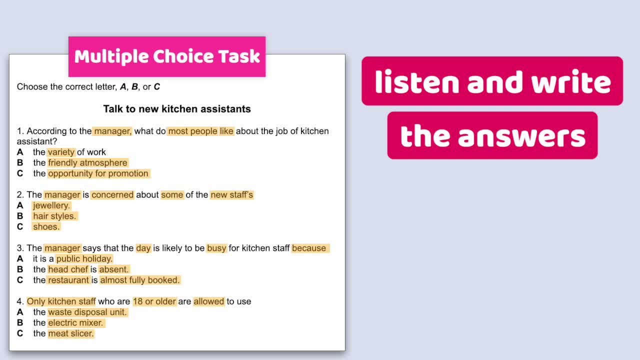 And I'll tell you straight away that if you do well, we might think about moving you up and giving you some more responsibility. Right, Well, you've all shown up on time, which is an excellent start. Now I'm glad to see none of you have unsuitable footwear. 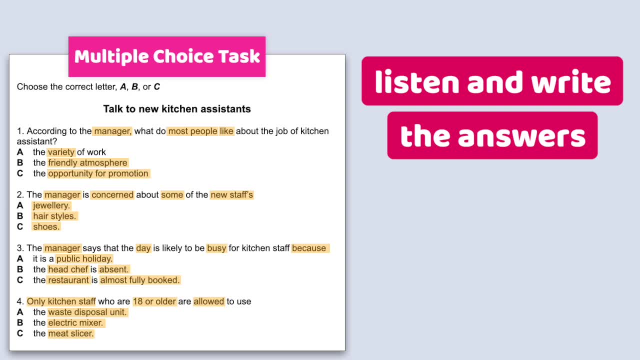 so that's good. You need to be careful, as the floors can get very wet and slippery. Those of you with long hair have got it well out of the way, but some of you will need to remove your rings and bracelets. Just put them somewhere safer today and remember to leave them at home. 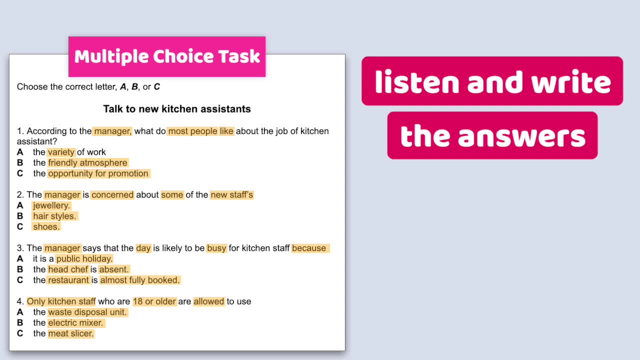 tomorrow, as they can be a safety hazard. Now it's going to be a busy day for you all today. We don't have any tables free for this evening and only a few for lunch. Fortunately, we've got our head chef back. He was away on holiday. He's going to be here for a while, So 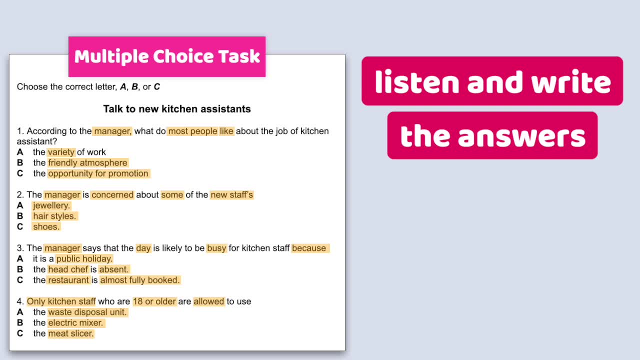 last week, which meant the other chefs had extra work. Now I'll tell you a bit more about the job in a minute, but first some general regulations For all of you, whatever your age. there's some equipment you mustn't use until you've been properly trained, like the waste disposal system. 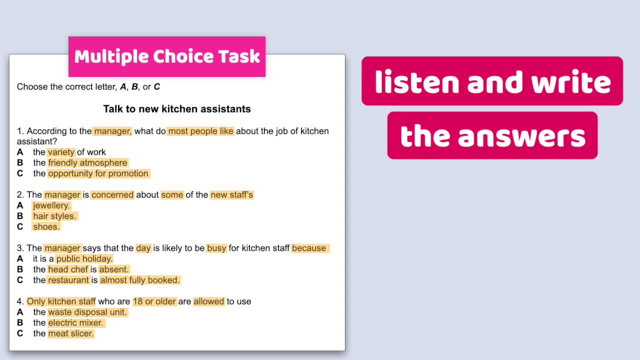 for example for health and safety reasons. Then I think there are two of you here who are under 18, That's Emma and Jake, isn't it Right? So for you two, the meat slicer is out of bounds. And, of course, none of you are allowed to use the electric mixer until you've been shown how it. 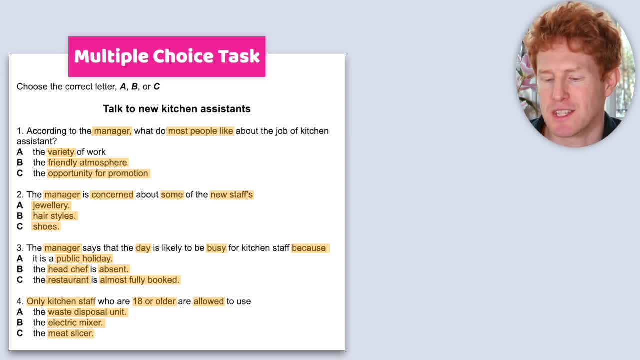 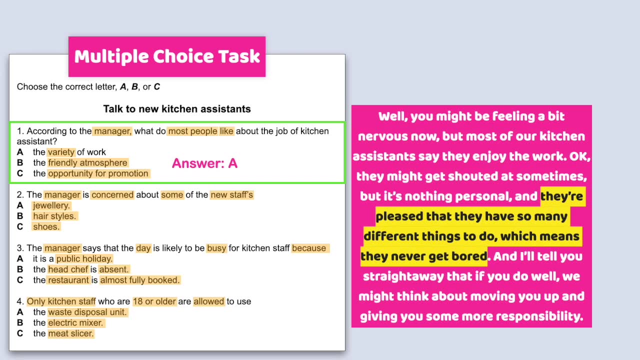 works. Okay, let's look at the answers together. So number one: the answer is A Listen again. Well, you might be feeling a bit nervous now, but most of our kitchen assistants say they enjoy. Okay, they might get shouted at sometimes, but it's nothing personal And they're pleased that. 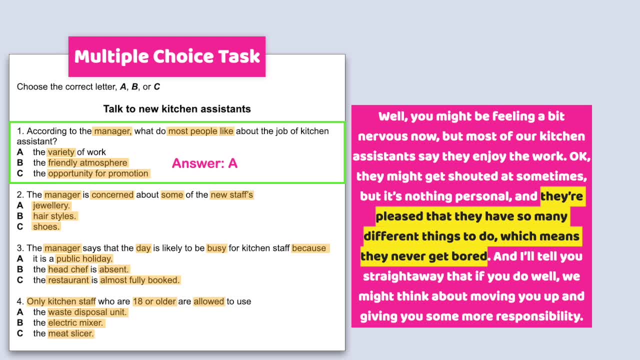 they have so many different things to do, which means they never get bored, And I'll tell you straight away that if you do well, we might think about moving you up and giving you some more responsibility. Okay, the answer is A, because the speaker said they are pleased that they have. 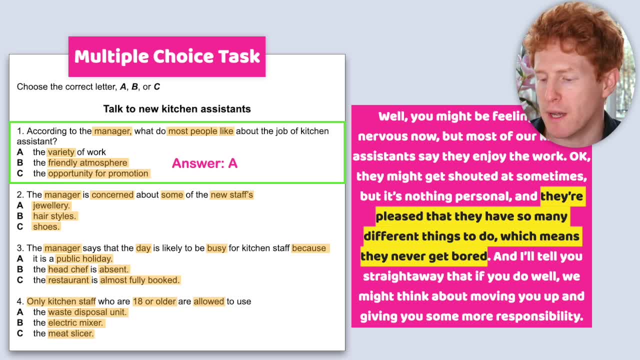 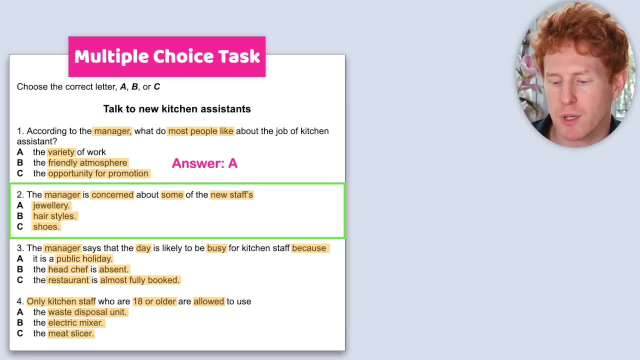 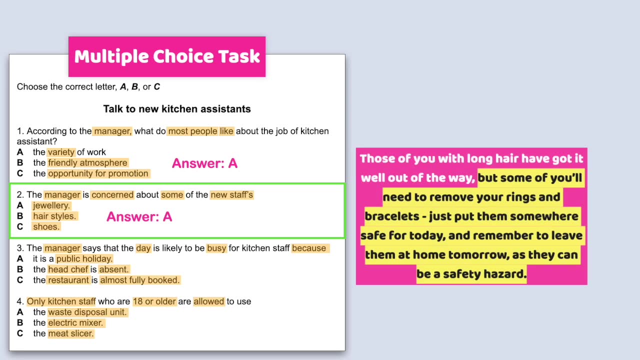 so many different things to do, So different roles, which means they never get bored. Okay, number two. The answer is A. Listen again. Those of you with long hair have got it well out of the way, but some of you will need to remove. 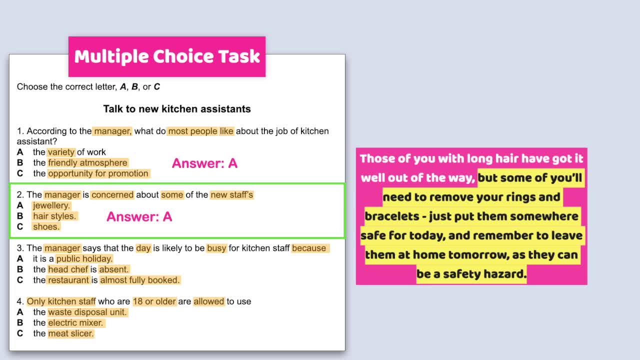 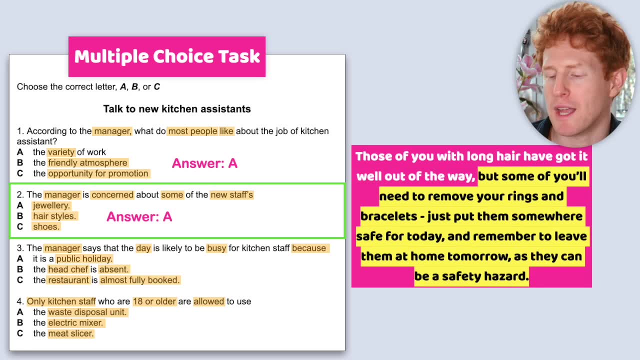 your rings and bracelets. Just put them somewhere safe for today and remember to leave them at home tomorrow, as they can be a safety hazard. Okay, the speaker says you need to remove your rings and bracelets. So rings and bracelets are pieces of jewellery. The speaker is concerned or worried? 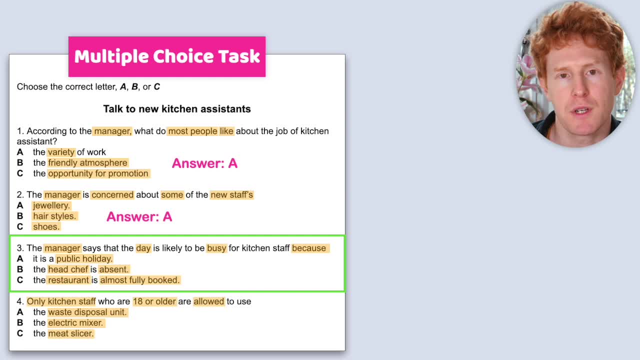 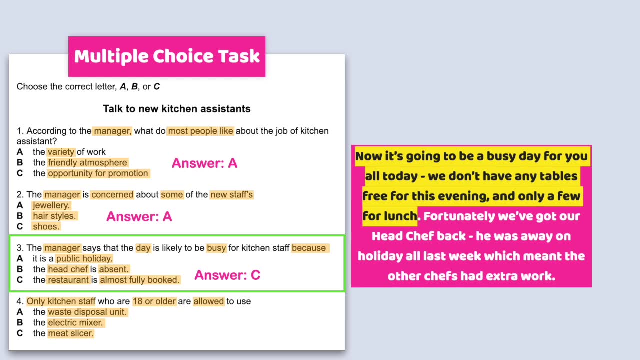 about this jewellery Number three? The answer is C. Listen again Now. it's going to be a busy day for you all today. We don't have any tables free for this evening And only a few for lunch. Fortunately, we've got our head chef back. He was away on holiday all. 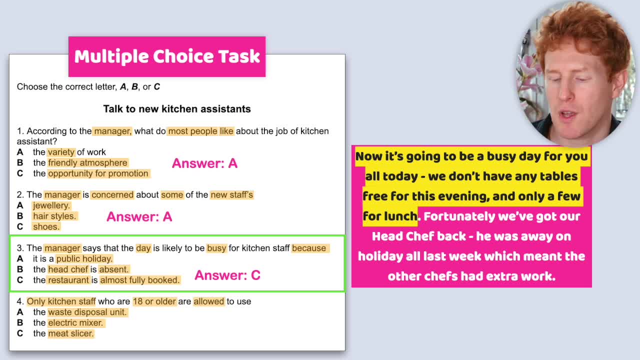 last week, which meant the other chefs had extra work. Okay, this was a tricky one. The speaker said we don't have any tables free for this evening and only a few for lunch. So the restaurant is fully booked for the evening and there are only a few tables that are free for. 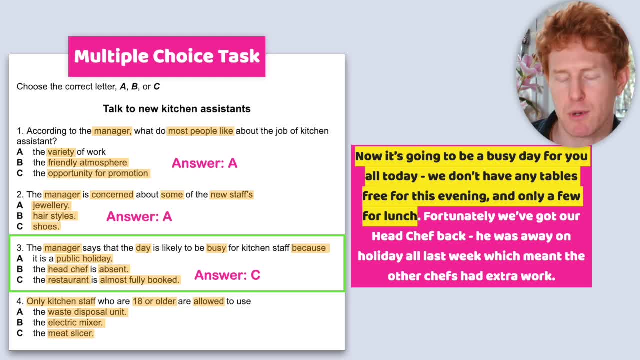 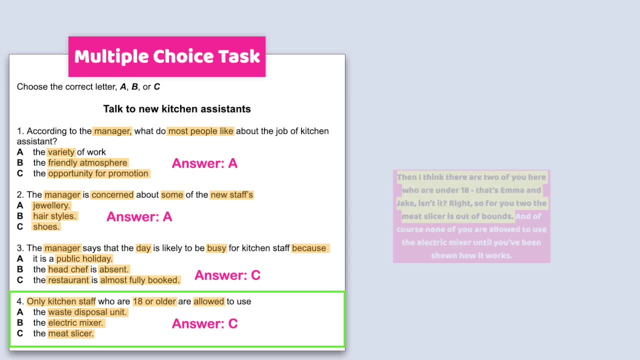 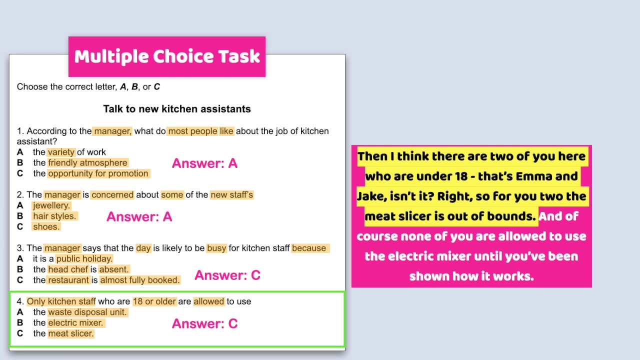 lunch, So the restaurant is almost fully booked. Number four: The answer is C. Listen again, Then I think there are two of you here who are under 18.. That's Emma and Jake, isn't it Right? So for you two, the meat slicer is out of bounds. And, of course, 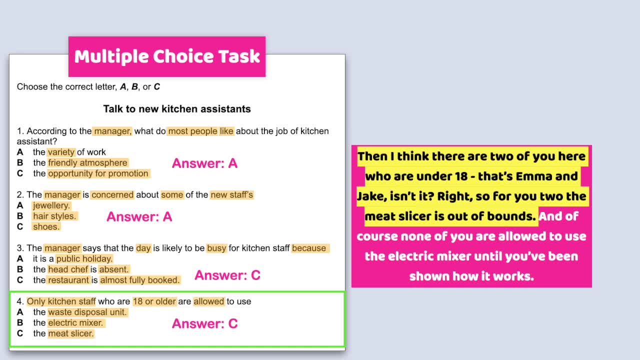 none of you are allowed to use the electric mixer until you've been shown how it works. Okay, So the speaker identifies two people that are under 18, Emma and Jake, and then this person says to Jake and Emma: the meat slicer is out of bounds. So out of bounds means you cannot go to. 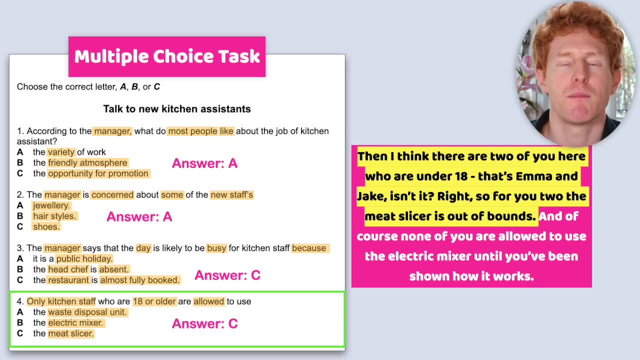 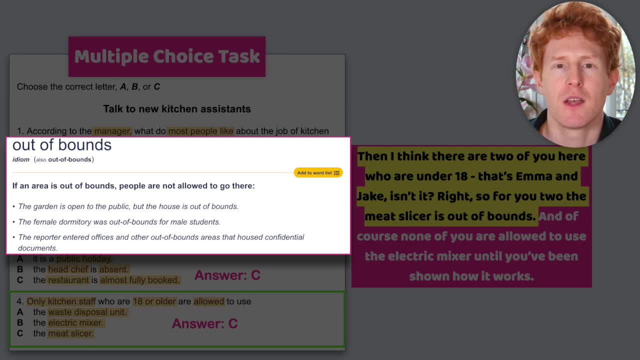 this place or you cannot use this machinery. It is not permitted for you to use it, It is out of bounds. For example, you might say to your child: while I'm cooking, I'm going to make a meat slicer, So I'm going to have to have a meat slicer, And then the sleeper is going to say to the child: 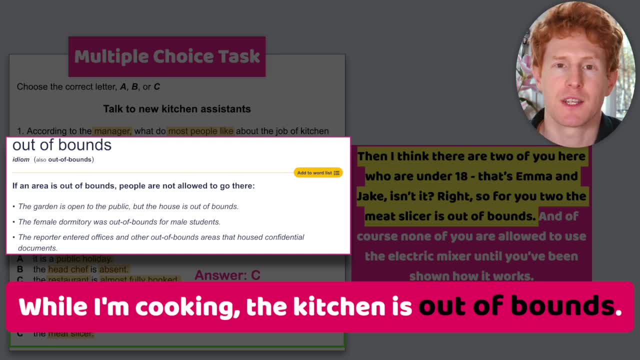 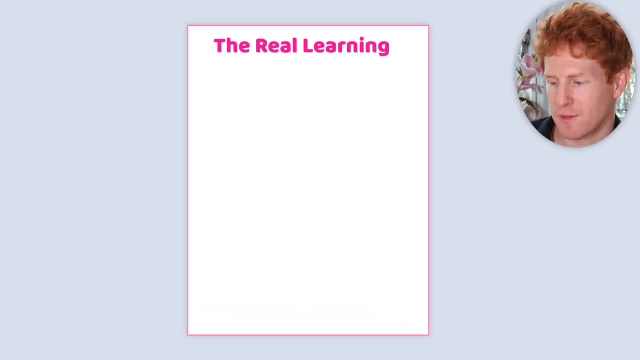 While I'm cooking. the meat slicer is out of bounds, So I'm not allowed to use the electric mixer. The kitchen is out of bounds, which means your child cannot enter the kitchen while you are cooking. Okay, now here comes the real learning. 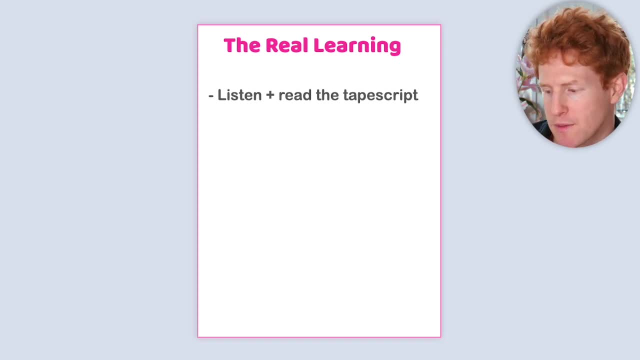 Now you're going to listen and read the tape script Afterwards. you're going to go over the questions you got wrong. You're going to make a note of some new vocabulary that you have learned today. You're going to recap what you have learned from today. 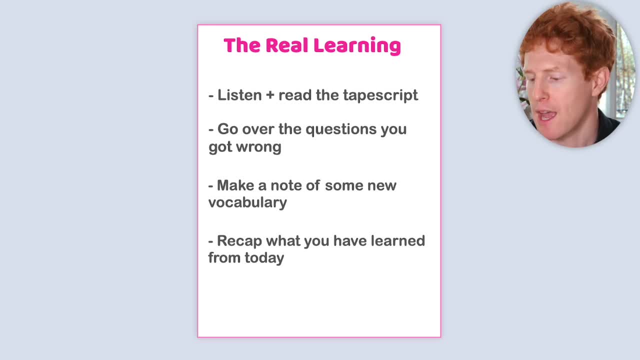 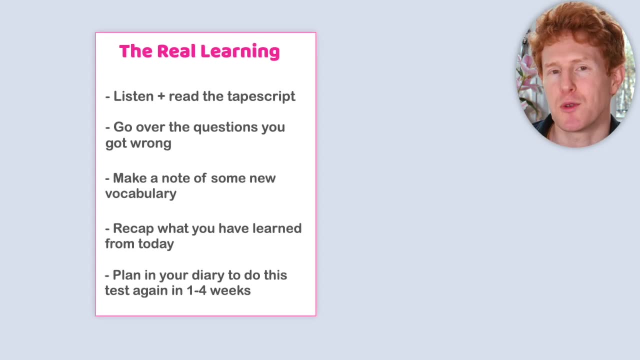 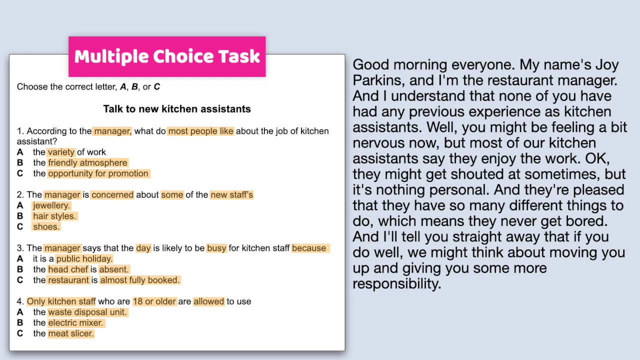 for example, maybe a new strategy or skill, And then you're going to plan in your diary to do this test again in one to four weeks. Okay, time to listen and read. Good morning everyone. My name's Joy Parkins and I'm the restaurant manager. 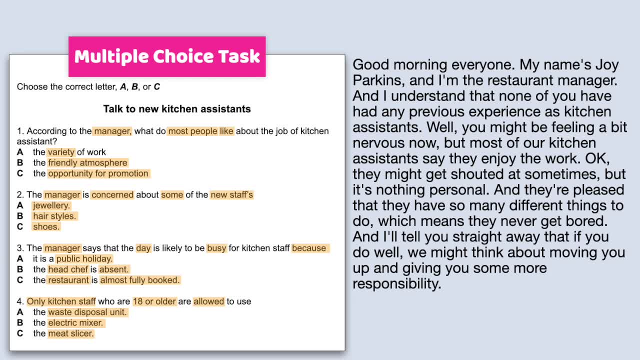 And I understand that none of you have had any previous experience as kitchen assistants. Well, you might be feeling a bit nervous now, but most of our kitchen assistants say they enjoy the work. Okay, they might get shouted at sometimes, but it's nothing personal. 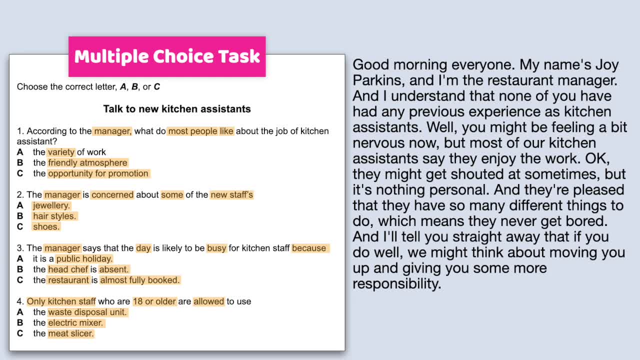 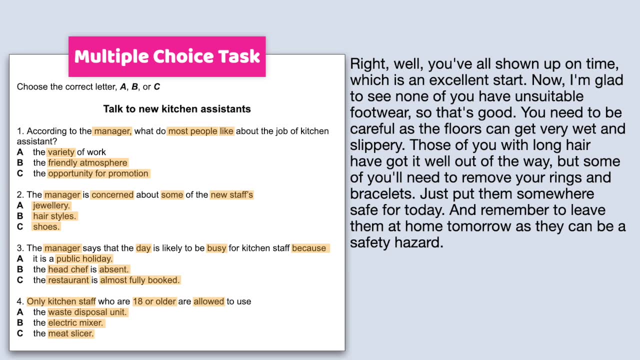 And they're pleased that they have so many different things to do, which means they never get bored. And I'll tell you straight away that, if you do well, we might think about moving you up and giving you some more responsibility, Right? well, you've all shown up on time. 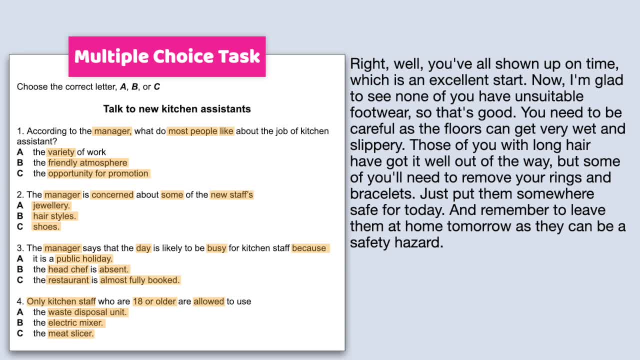 which is an excellent start. Now, I'm glad to see none of you have unsuitable footwear, so that's good. You need to be careful, as the floors can get very wet and slippery. Those of you with long hair have got it well out of the way. 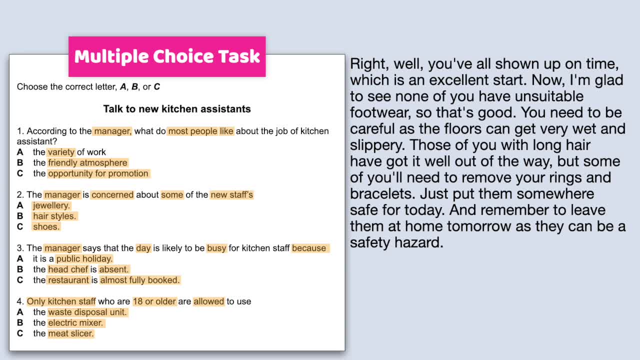 but some of you will need to remove your rings and bracelets. Just put them somewhere safe for today And remember to leave them at home tomorrow, as they can be a safety hazard. Now. it's going to be a busy day for you all today. 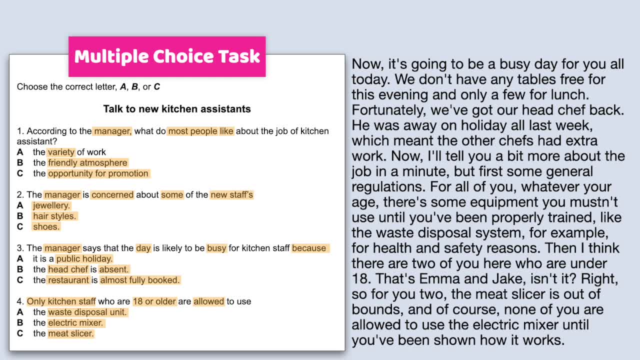 We don't have any tables free for this evening and only a few for lunch. Fortunately, we've got our head chef back. He was away on holiday all last week, which meant the other chefs had extra work. Now I'll tell you a bit more about the job in a minute.